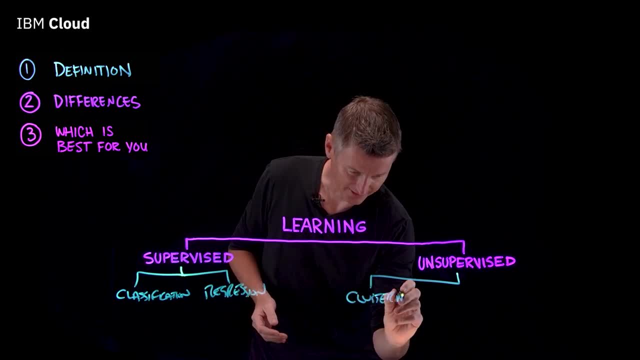 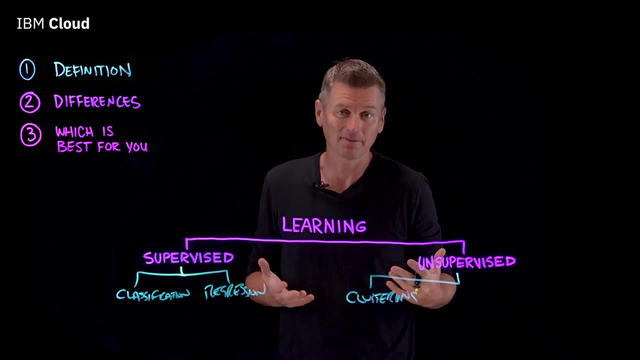 and dimensionality reduction. So let's take a look at each one of those, Starting with clustering Now. clustering is where the algorithm groups similar experiences together. So a common application of clustering is customer segmentation, where businesses might group customers together based on similarities like I don't know age or location, you know states, age, sectors, brands. 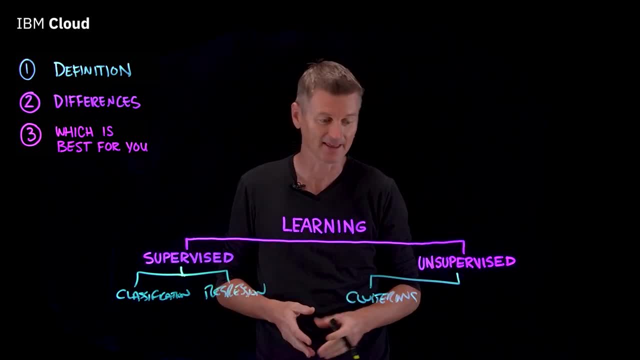 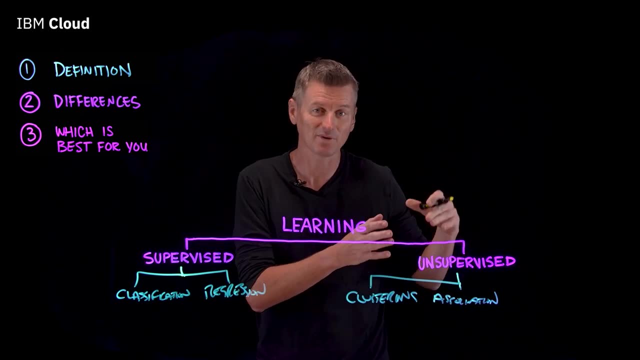 origins, governments, etc. They're not all changing. You can use their management method to give you a historic value or location or spending habits, something like that. Then you have association, and association is where the algorithm looks for relationships between variables in the data. Now association: 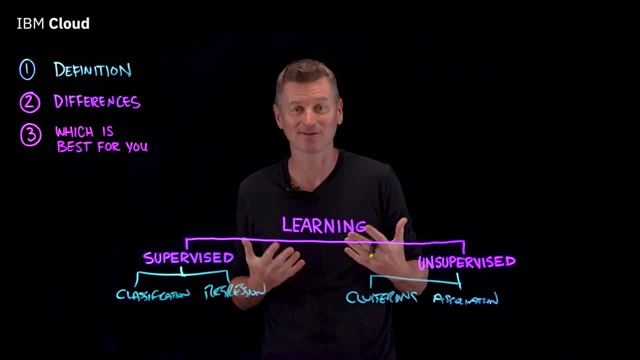 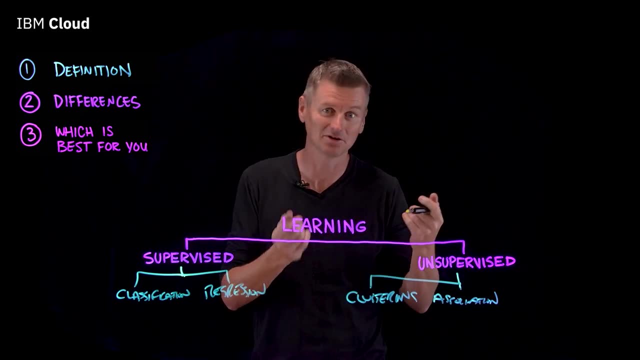 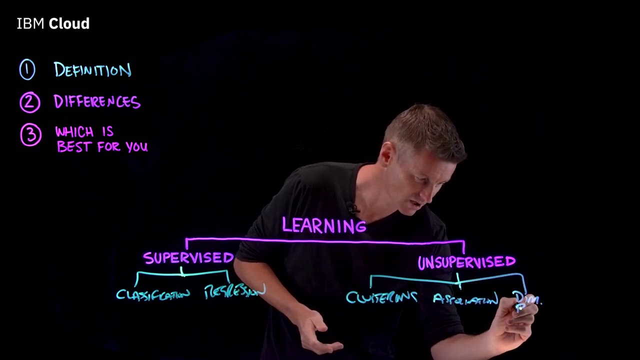 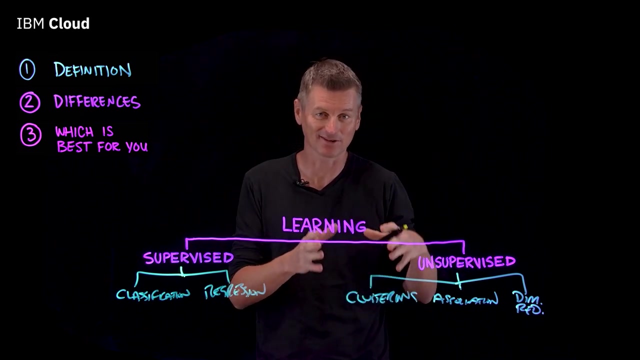 rules are often used in market basket analysis, where businesses want to know which items are often bought together. You know something along the lines of customers who bought this item also bought that sort of thing. The final one to talk about is dimensional reduction, and this is where the algorithm reduces the number of variables in the data, while still 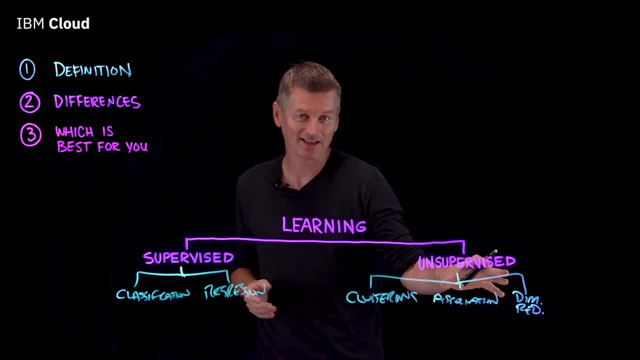 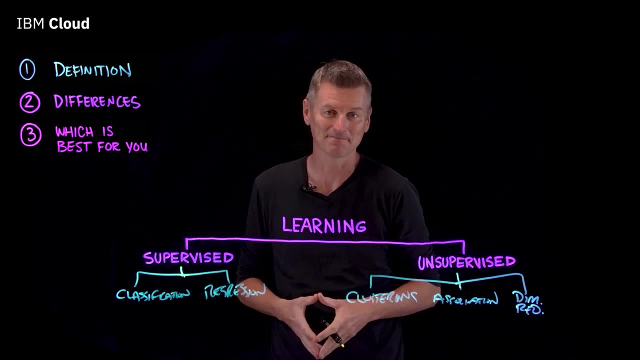 preserving as much of the information as possible. Now, often this technique is used in the pre-processing data stage, such as when auto encoders remove noise from visual images to improve picture quality. Okay, so let's talk about the differences between these two types of learning. 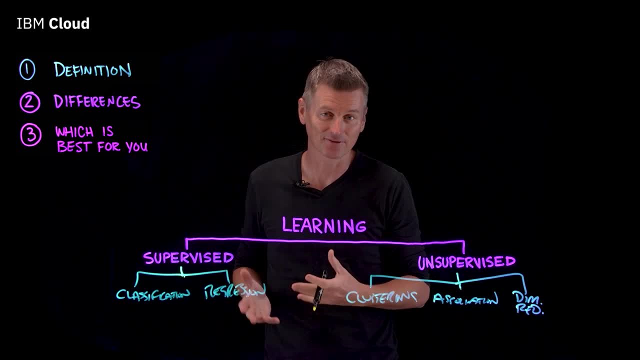 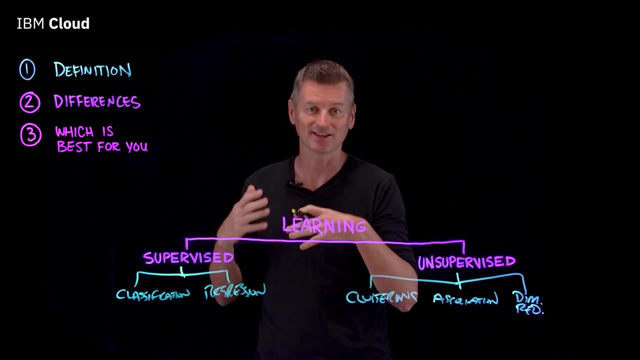 In supervised learning, the algorithm learns from training data sets by iteratively making predictions on the data and then adjusting for the correct answer. While supervised learning models tend to be more accurate than unsupervised learning models, they do require all of this upfront human intervention to label the data appropriately. For example, a supervised learning 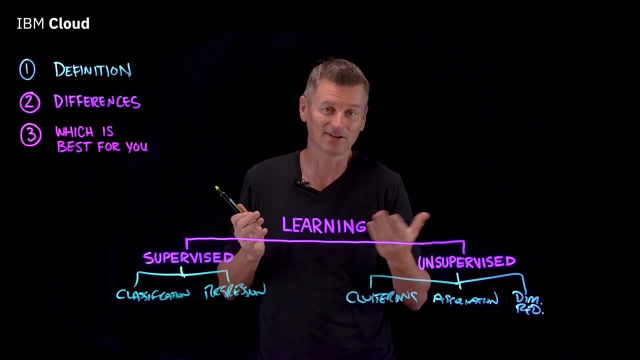 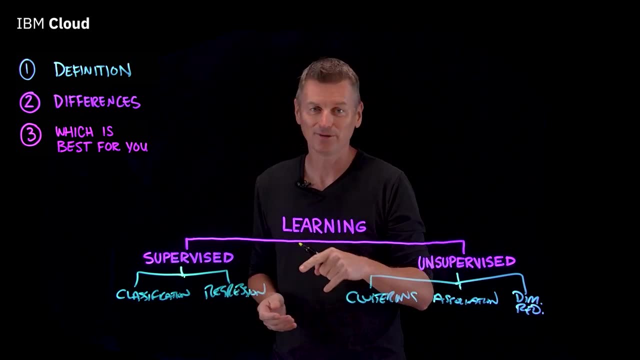 model can predict how long your commute will be, on the time of day and thinking about the weather conditions and so forth, But first you'll have to train it to know things like rainy weather extends the driving time. By contrast, unsupervised learning models work on their own to discover the inherent structure of 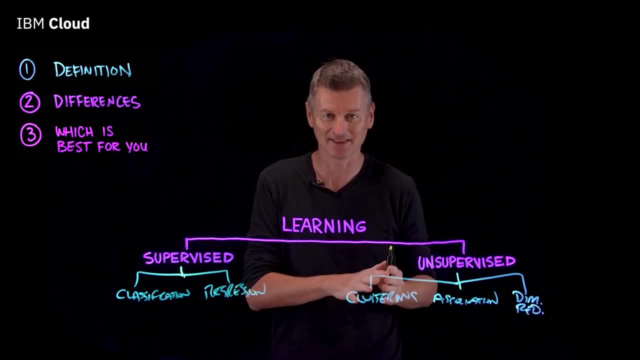 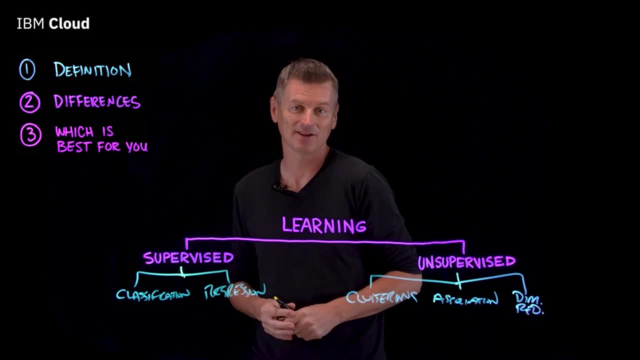 unlabeled data. These models don't need humans to intervene. They can automatically find patterns in data and group them together. So, for example, an unsupervised learning model can cluster images by the objects they contain, Things like people and animals and buildings. 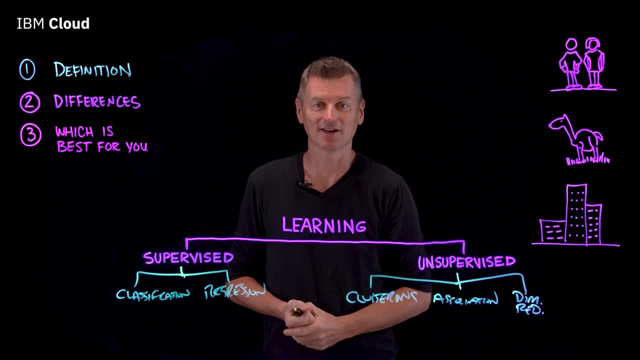 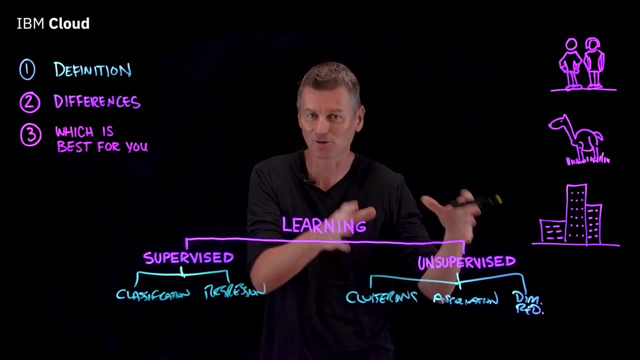 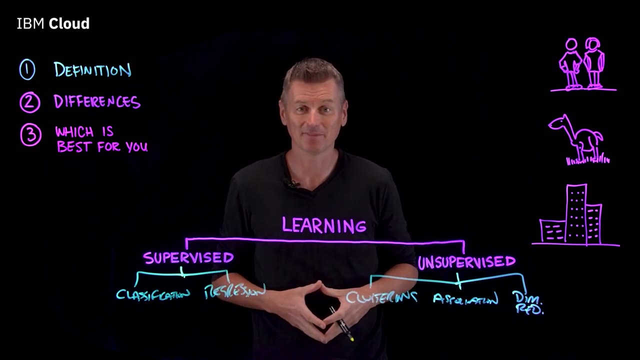 Without being told what those objects were ahead of time. Now an important distinction to make is that unsupervised learning models don't make predictions. They only group data together. So if you were to use an unsupervised learning model on that same commute data set, it would group together commutes with similar conditions like the time. 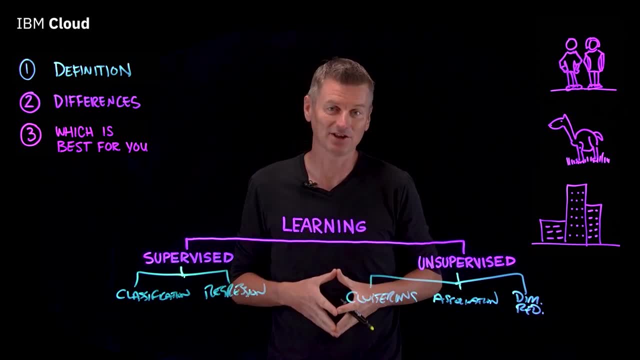 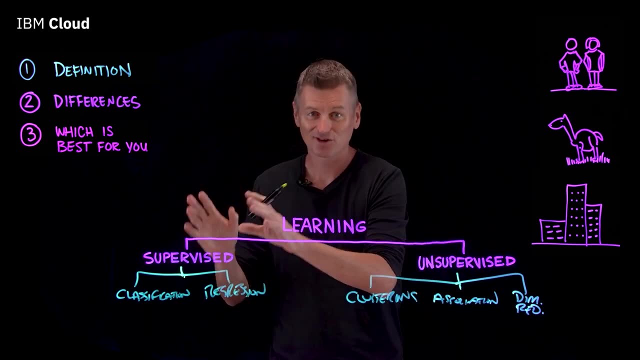 of day and the weather, But it wouldn't be able to predict how long each commute would take. Okay, so which of these two options is right for you? In general, supervised learning is more commonly used than unsupervised learning, And that's really because 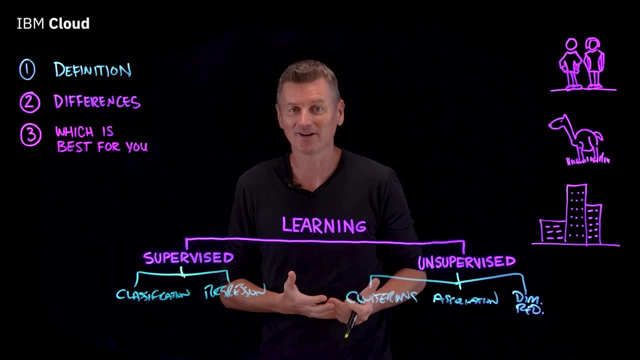 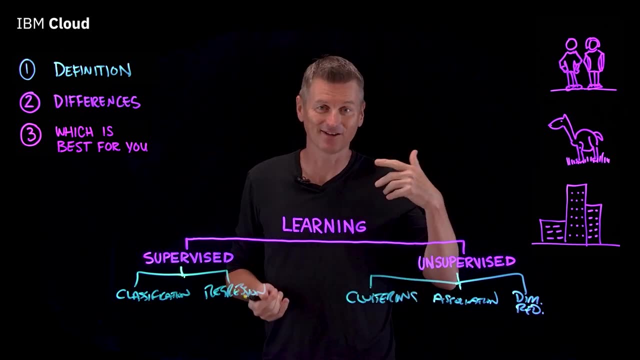 it's more accurate and efficient. but, that being said, unsupervised learning has its own advantages. There's two I can think of. Firstly, unsupervised learning can be used on data that is not labeled, which is often the case in real world data sets. And then, secondly, unsupervised learning can be 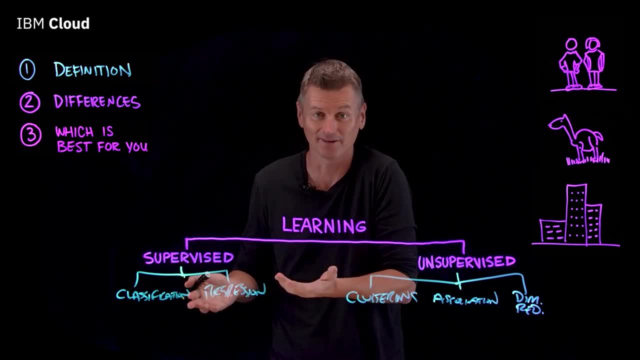 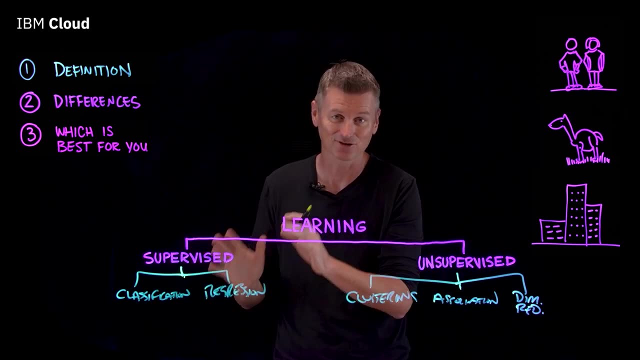 used to find hidden patterns in data that supervised learning models just wouldn't find. Classifying big data can be a real challenge in unsupervised learning, but the results are highly accurate and trustworthy and, in contrast, unsupervised learning can handle large volumes of data in real time, But there's a lack of 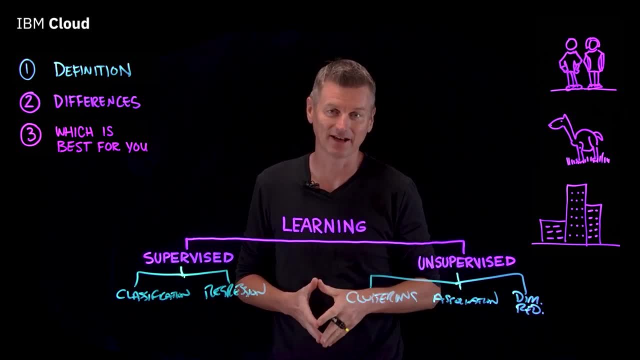 transparency into how that data is clustered and a higher risk of inaccurate results. But wait, it is not an either or choice. May I present to you the middle ground, known as semi-supervised learning. This is a happy medium where you use a training data set with 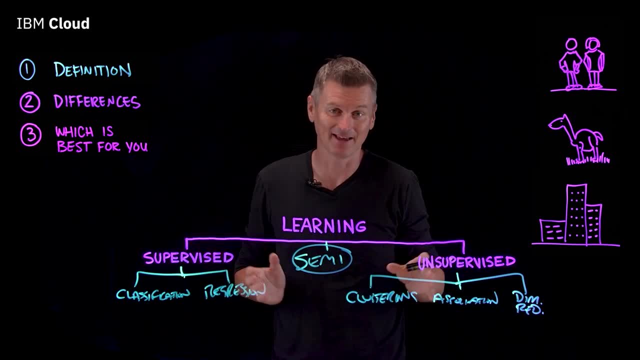 both labeled and unlabeled data, and it's particularly useful when it's difficult to extract relevant features from data and when you have a high volume of data. So, for example, you could use a semi-supervised learning algorithm on a data set with millions of images, where only 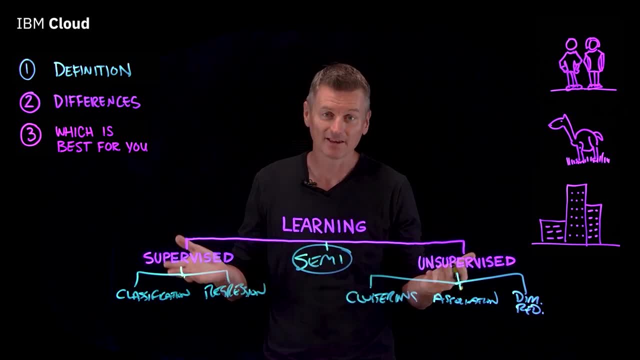 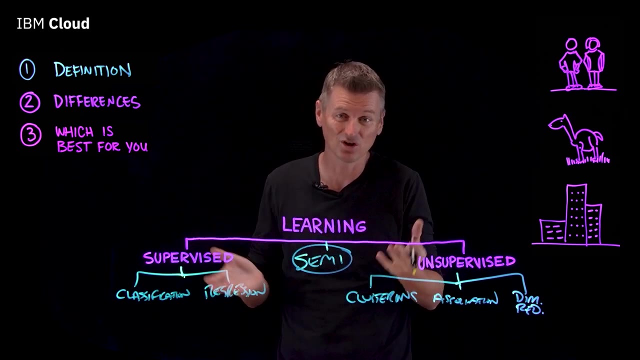 a few thousand of those images are actually labeled Semi-supervised learning. Semi-supervised learning, Semi-supervised learning, Optimized learning, is ideal for medical images, where a small amount of training data can lead to a significant improvement in accuracy. For example, a radiologist can look at and label some small subset of CT scans for tumors.